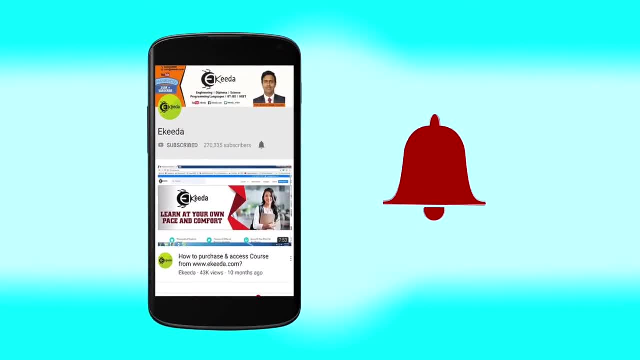 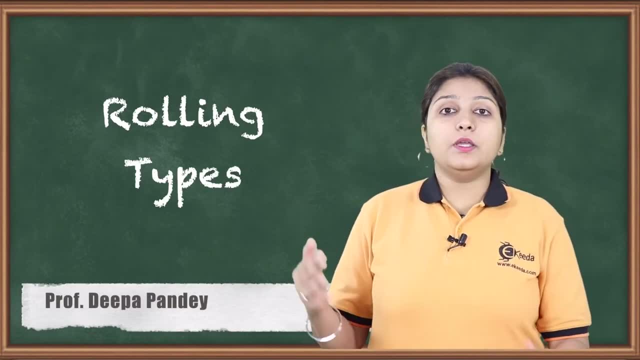 Click the bell icon to get latest videos from eKIDA. Hello friends, today we are going to see what is rolling and what are its type. How rolling is carried out are different ways in different stands, And what are the stands on which rolling is carried out. we are going to see in this video. 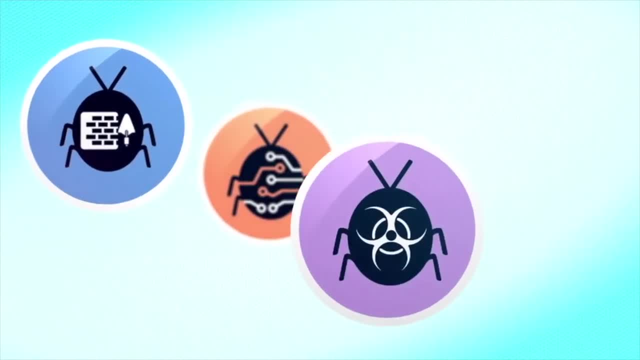 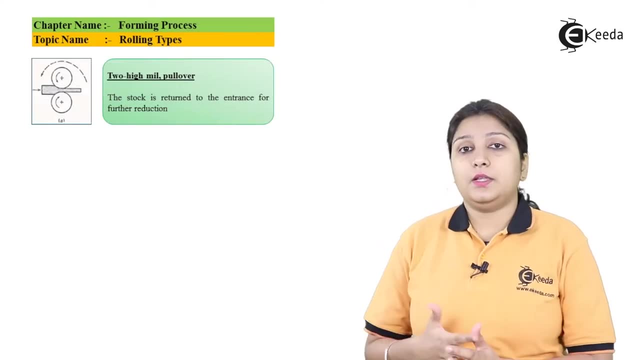 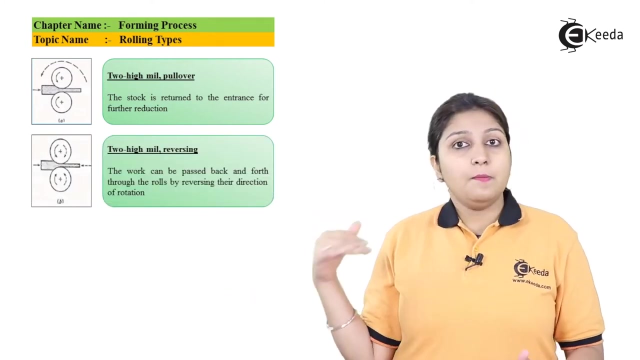 So basically, on the screen, different types of stands are being placed. There are basic 5 types of stands. Also there are more types of stands, But we will talk about that one by one. In the first picture it is shown 2 high stands. 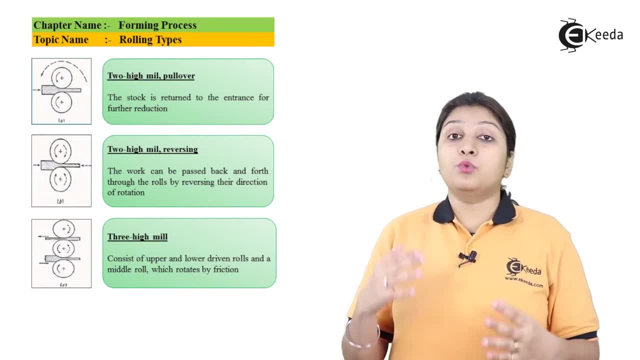 So basically I will clear what is a stand. Stand has some rollers Between which your material is passing. So material is passing through different rollers, But roller can't stand alone. They have to be kept properly aligned with each other. So for aligning that you need stands. 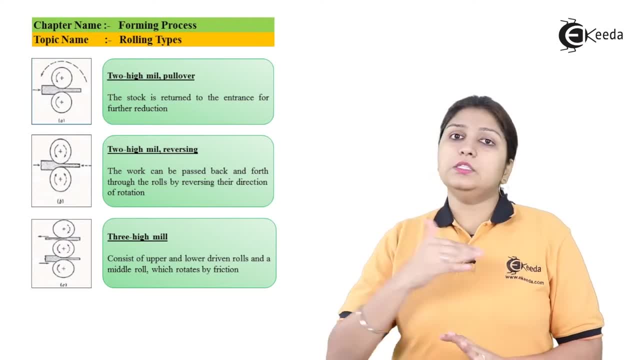 So the first type of stand is 2 high stand Which is going in a single direction. Like your roller is there, Material is passing through it in a single direction. The second type of stand is 2 high, but in a reverse direction. 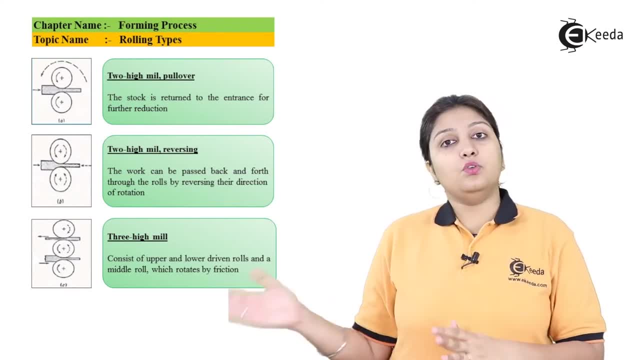 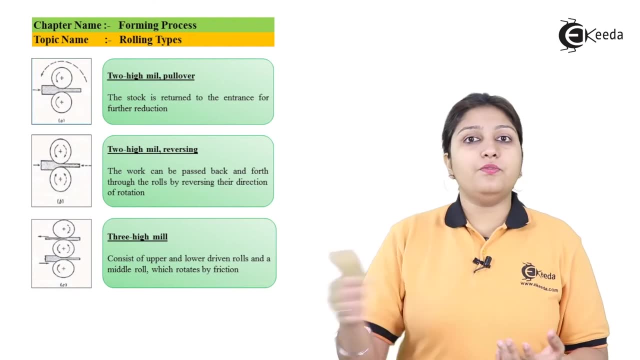 So the motion of the roller changes And the material goes in another direction. So the inlet would be different and the outlet would be different in both the cases, Like reversing and the front stand. But it is an example of a 2 high stand. 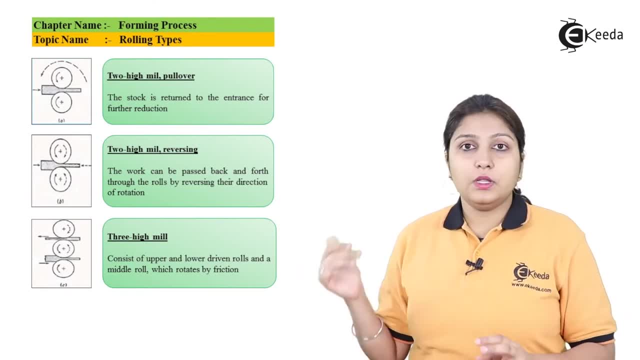 When we talk about 3 high stands. what is it shown is There are 3 kinds of rollers: First roller, last roller and a middle roller which is moving just due to friction, So your material can come through one direction and it can go through another direction. 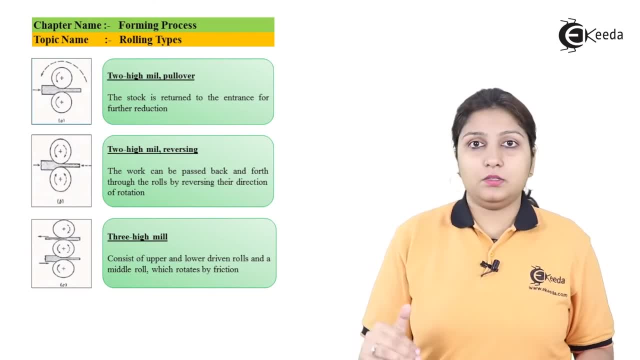 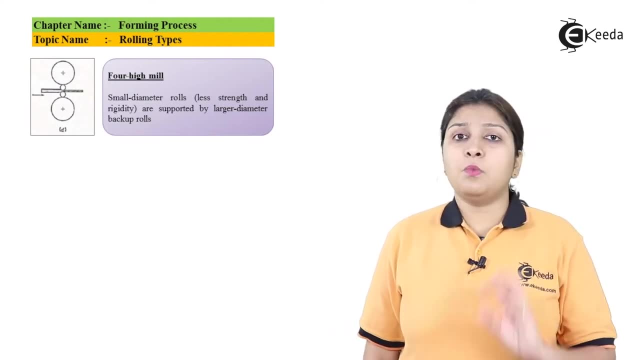 It can pass through Any number of rolling passes. Next is your 4 high stand. In the 4 high stand you can just see There are 2 small rollers like your planetary roller And 2 cluster rollers like your exact big rollers. 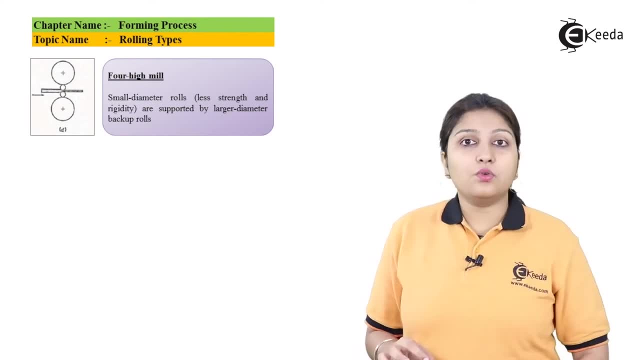 Your material is passed through 4 rollers. That's why the name is 4 high stand. So 2 rollers are small, just to give the support And just to give additional or excess reduction And the material is reduced Through a large amount in a 4 high stand. 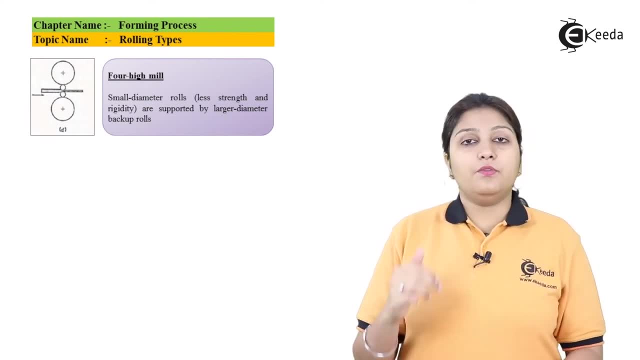 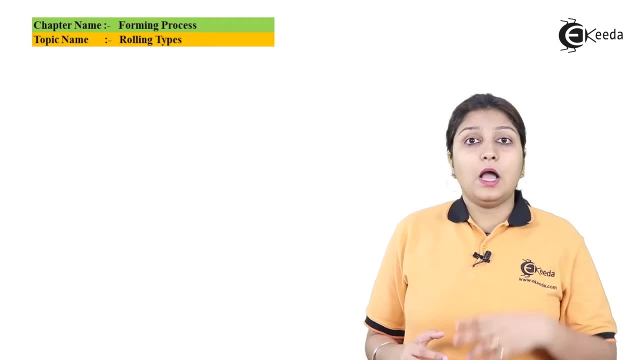 So after talking about 1,, 2,, 3 and 4 high stand, We will talk about cluster high stand. So in the diagram it is seen There are small clusters of planetary roll Above and beneath your exact material to be rolled. 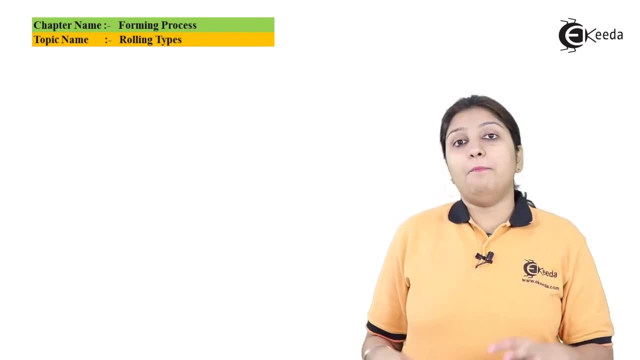 And also there are big rolls, So many rollers joined together And all the rollers enhance or advocates each other position. One rotates due to that, the other rotates, Third rotates, fourth rotates, and etc. So these all rollers rotate due to touching action. 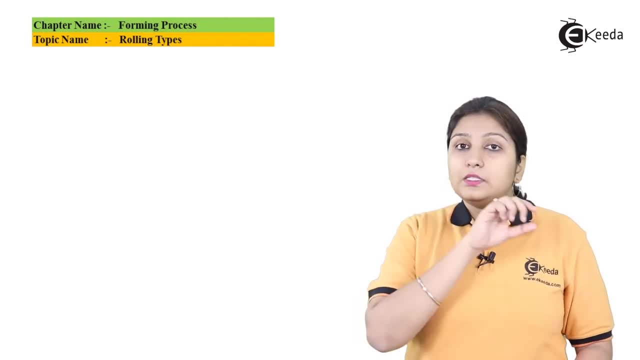 Or due to in contact with the other rollers And a single material is passed between them And again the reduction percentage of this roller is more So the material gets thin in a higher rate. So these are some 5 basic types of rollers. 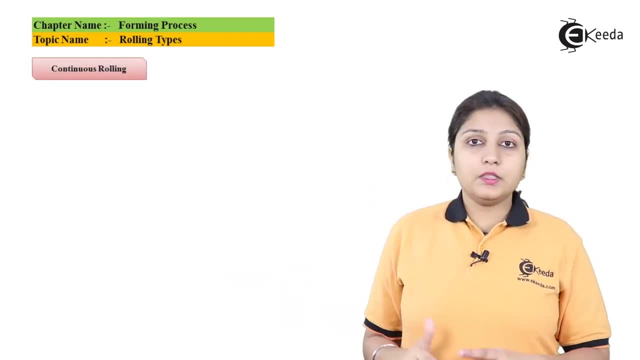 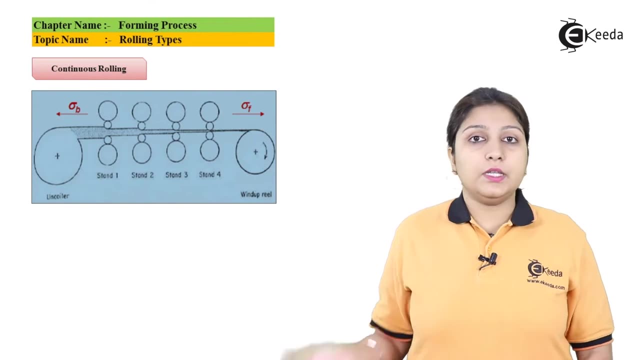 This is a continuous roller, So I will explain the diagram which is shown. There is an inlet, There is an outlet, You have different stands- How much it is needed? So different stands are there And rolling takes place at that stands. 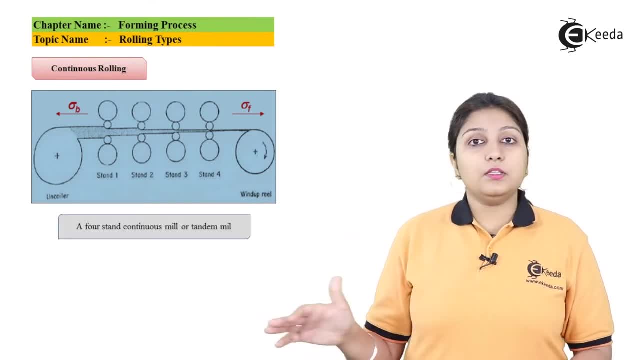 And your final product is made. So in this way, continuous process is done at a same speed. Your speed cannot be increased or decreased. If I will give an example of a label industry Where rollers are passing and making thin labels, There are n number of rollers through which your material passes. 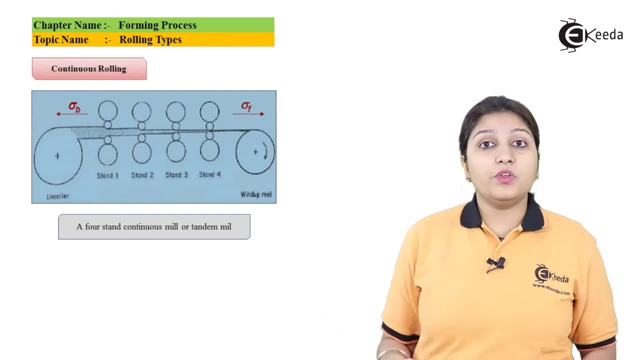 And there are different types of station on which your exact piercing takes place, Like your roll would be having your shape of the object Which is being parted or which is being subscribed on your object And it is passed to the next roller. Another object is there. 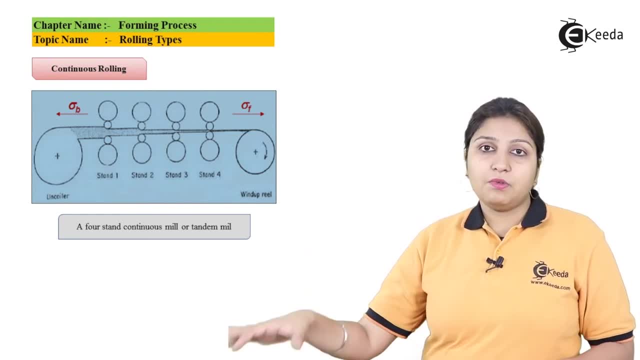 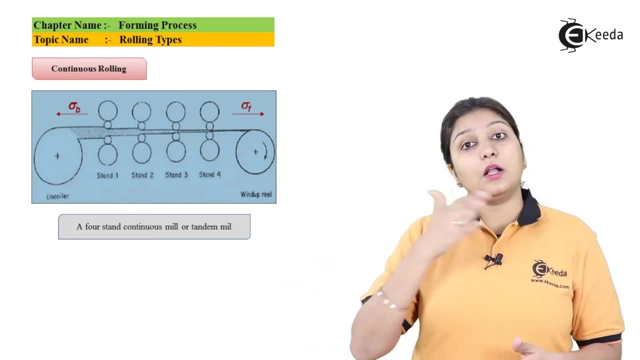 Like another thing can be done. Third, roller color can be filled or anything, But the impression on that object is done by your roller. So in this way a continuous stand can be used. This kind of roller is a planetary roller. You can see that it is a single cluster. 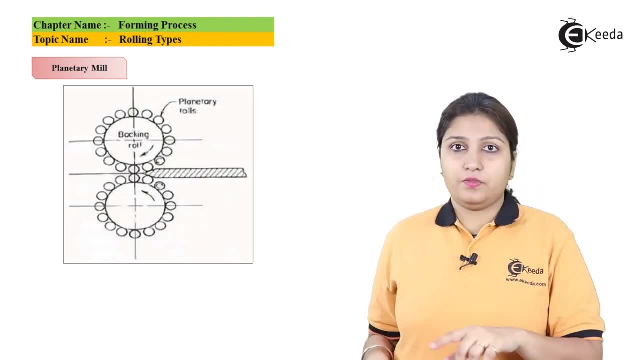 And above that, like in front of that, You can say around that there are more small rollers, Which helps in reducing your ingot or your slab in small blooms or a small sheet. So such kind of roller again enhances the reduction process, But both have to be at a same speed.